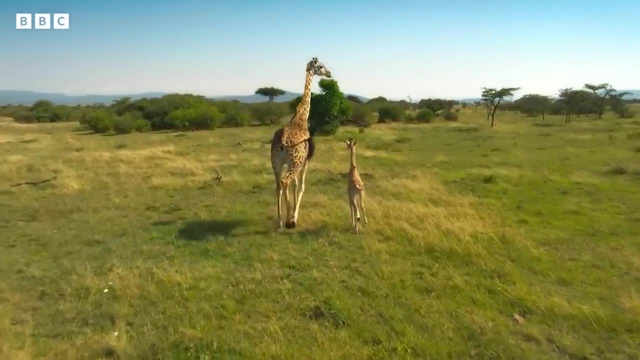 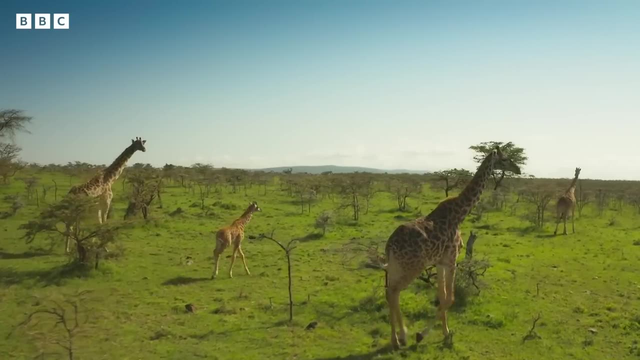 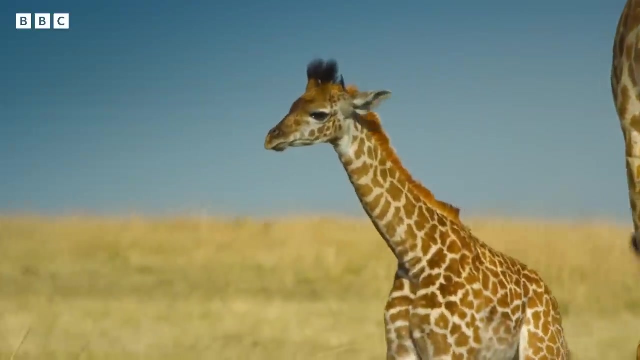 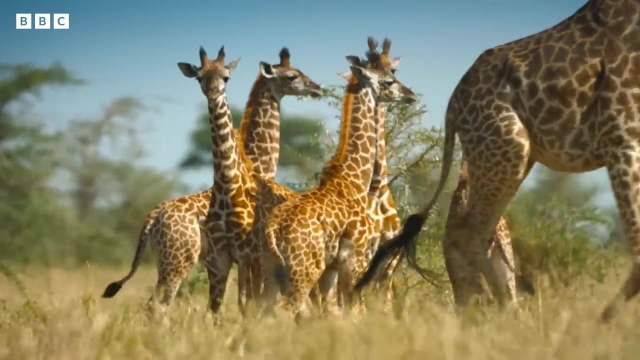 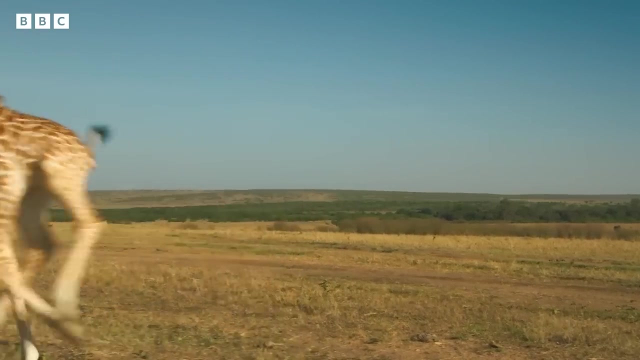 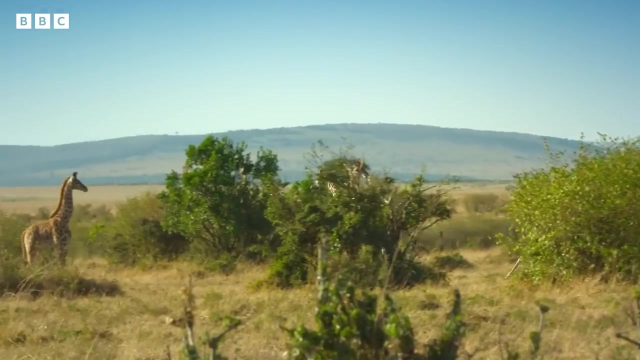 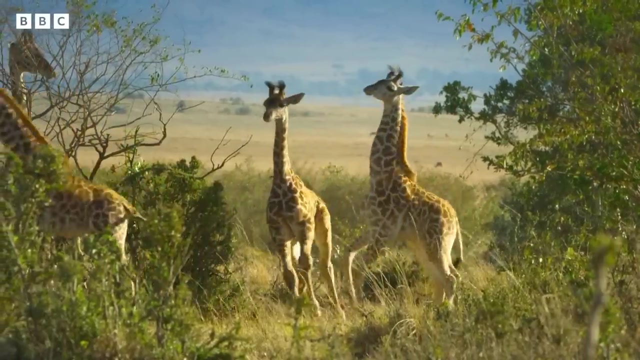 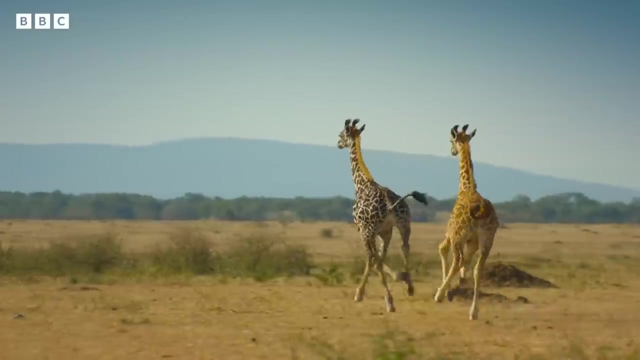 After his scare, Twigga stays close to his mother. But one taste of adventure is never enough. He'll make more friends if he can. It's never as hard as you think it might be, But when he's older it will be different. 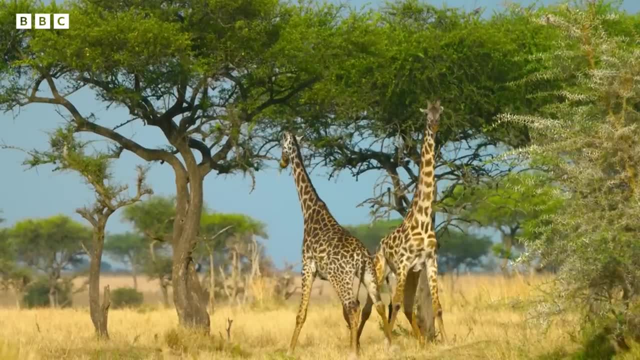 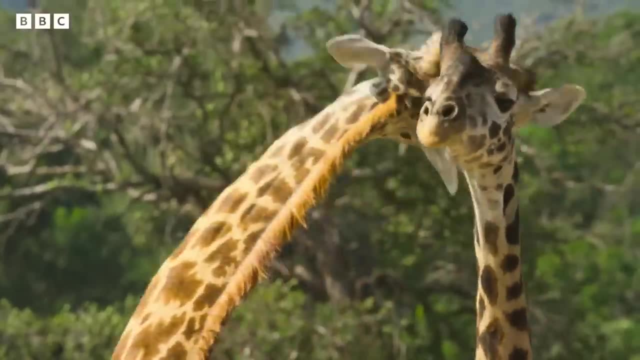 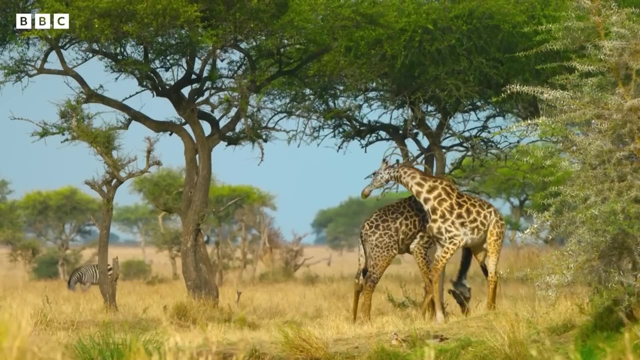 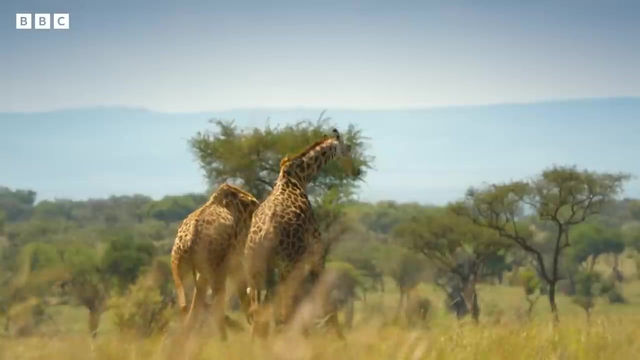 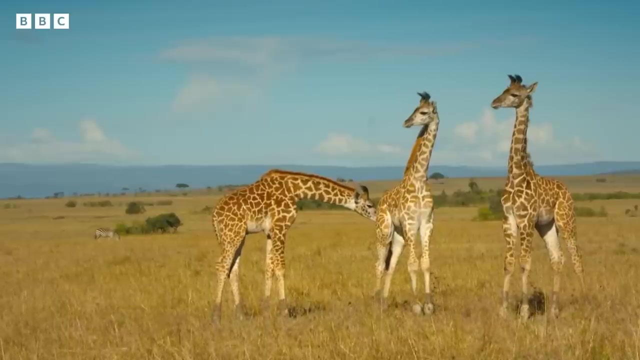 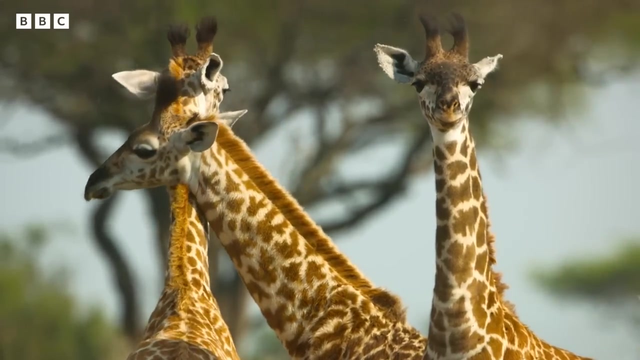 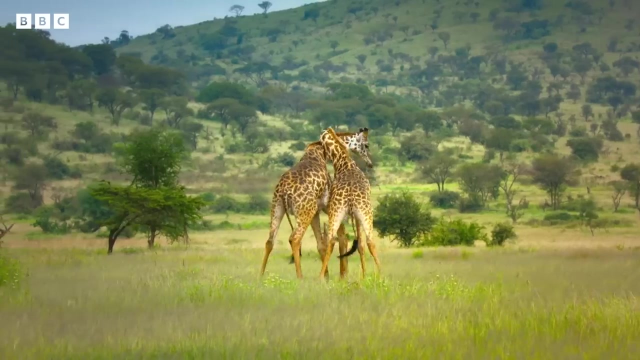 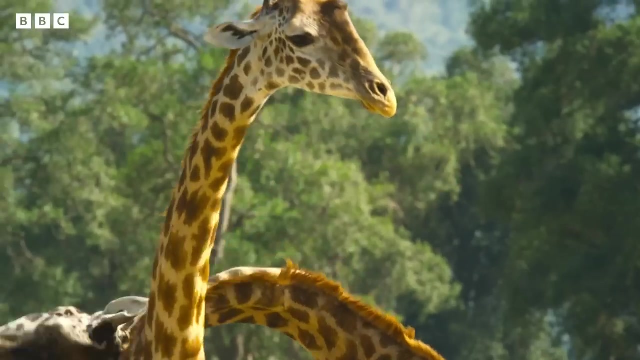 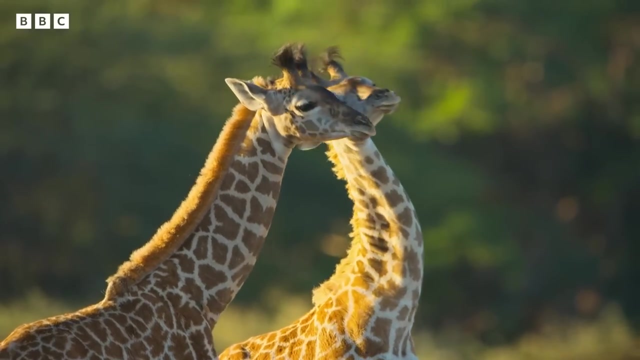 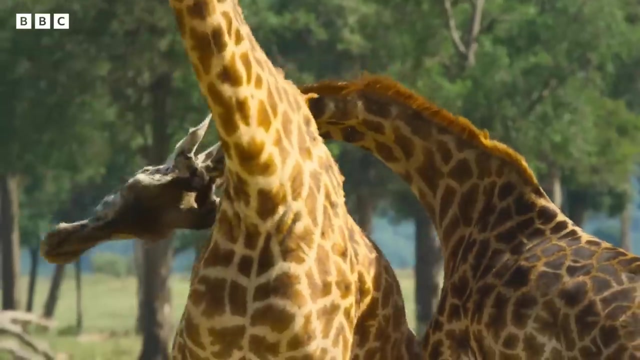 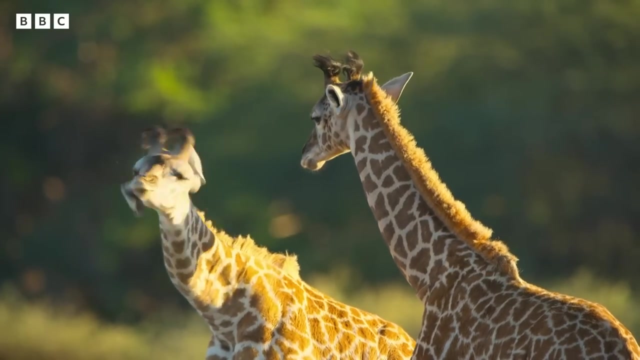 He'll meet rivals and have to defend himself. It's a glimpse into the future, But for now, future rivals are friends. Someone to practice with. Play fighting prepares them for the real battles ahead. Play on, play on. For now, though, it's just a game. 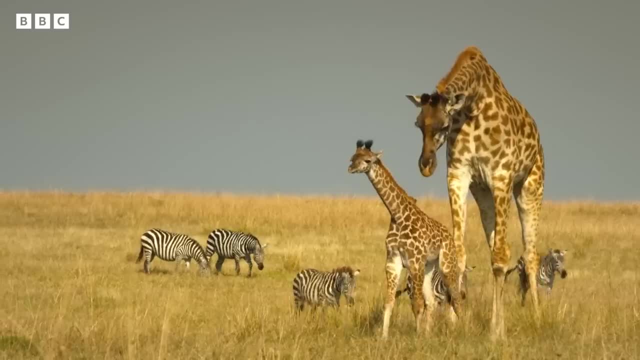 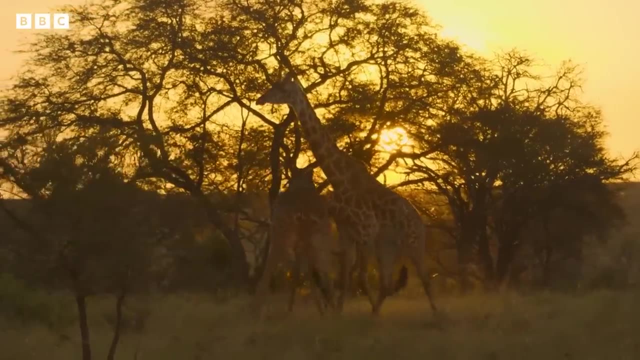 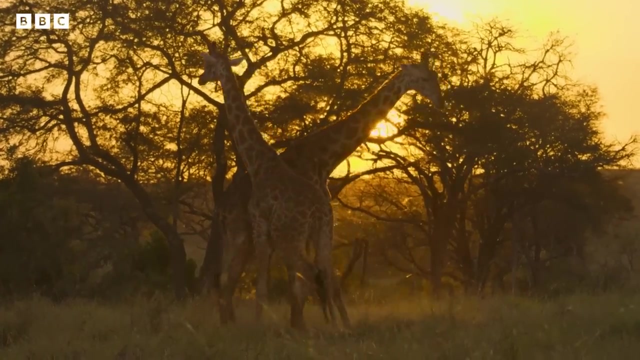 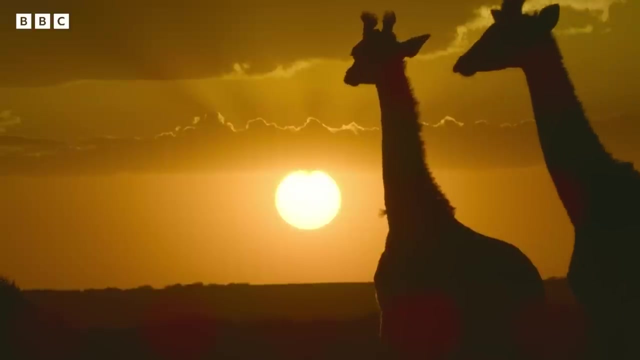 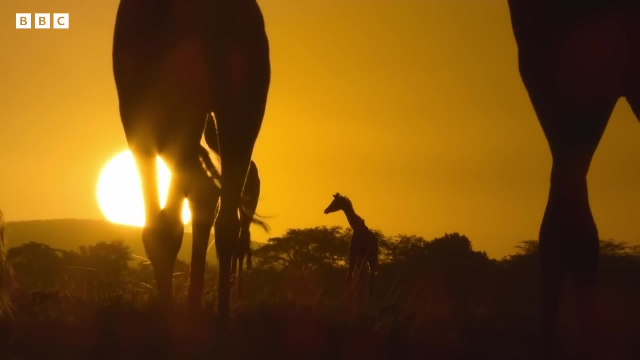 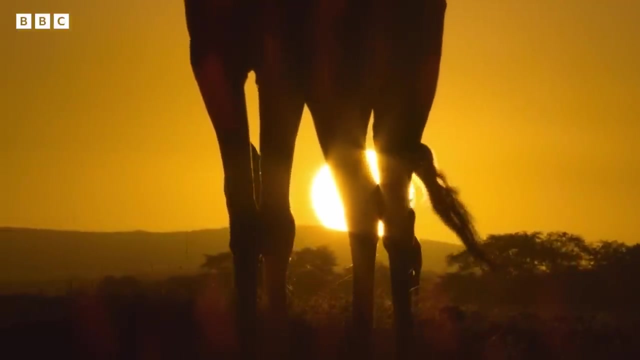 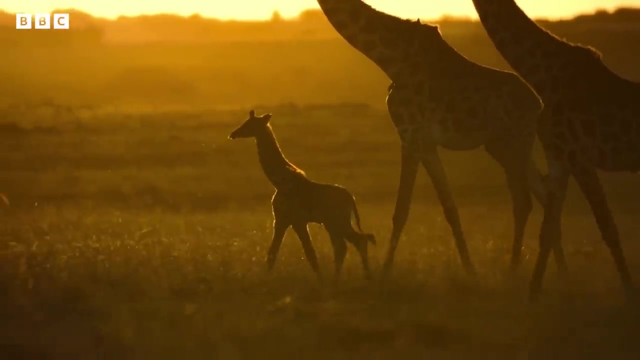 Even so, his mother keeps an eye on him. The fighting goes on into the night, while everyone else heads out to the plains. Twiggy's journey as a young giraffe is only just beginning, But he has all the support he'll ever need.